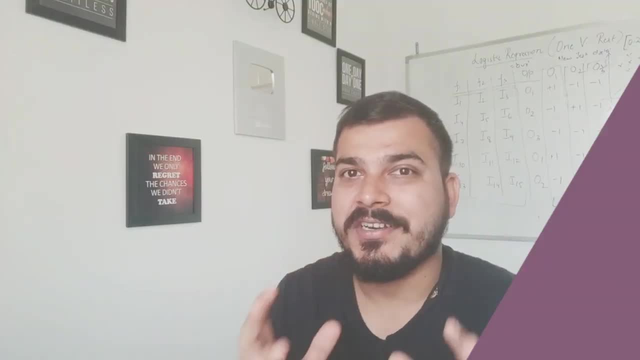 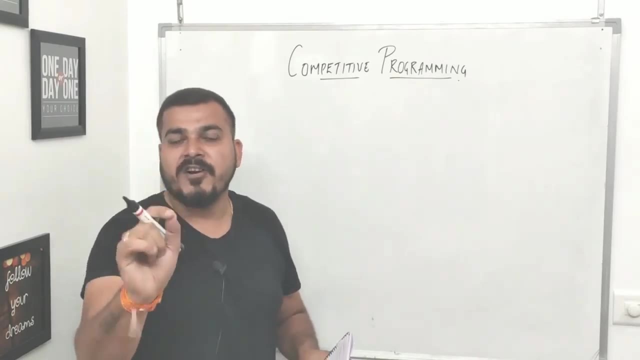 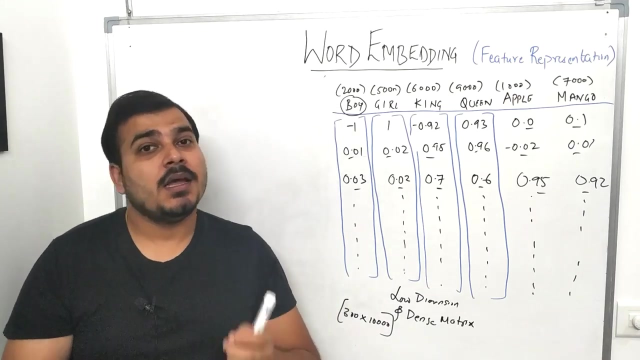 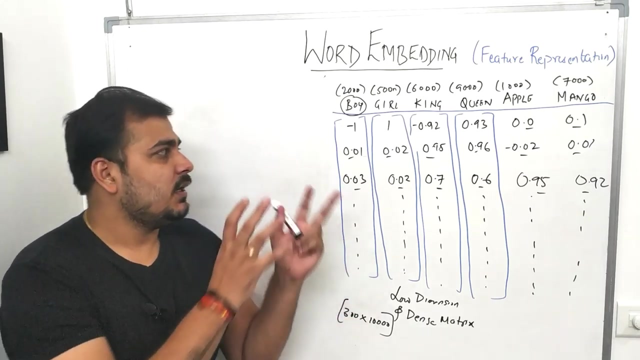 Hello, all my name is Krishnayak and welcome to my YouTube channel. So, guys, yesterday in my video, I had actually discussed about word embeddings. Now, in this particular video, we'll try to see how we can implement word embeddings with the help of embedding layers in Keras. Now, guys, I'm 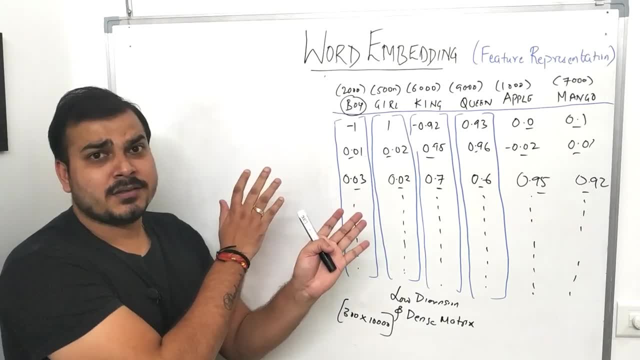 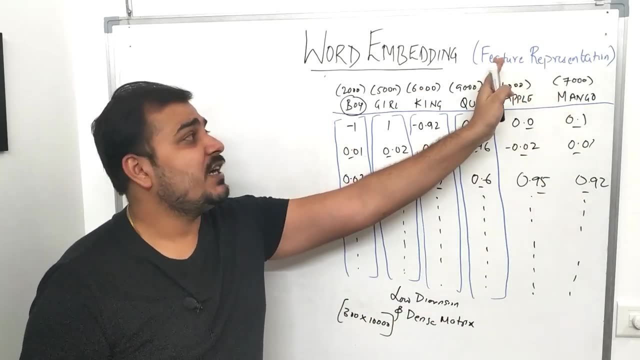 just going to explain you some theoretical stuff. hardly two minute theoretical stuff. then we'll move into the practical part. So you have already seen this kind of matrix, or the embedded matrix. we can also say it as the feature representation vectors with respect to each and every word. 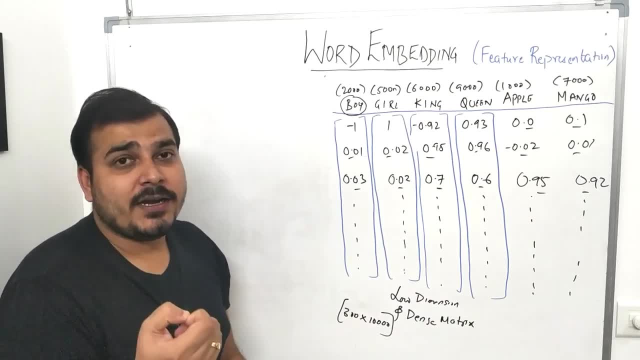 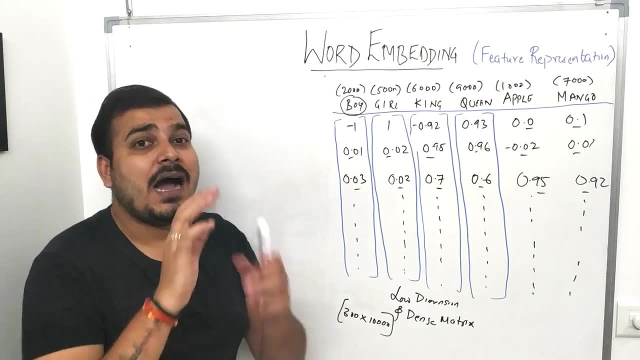 but how is this actually getting created? Okay, I had explained you about that, also based on some features in the left hand side, but when we are using embedding layer in Keras, the first thing how it actually works, Now understand. you have a sentence: the boy is good. Suppose. this is the. 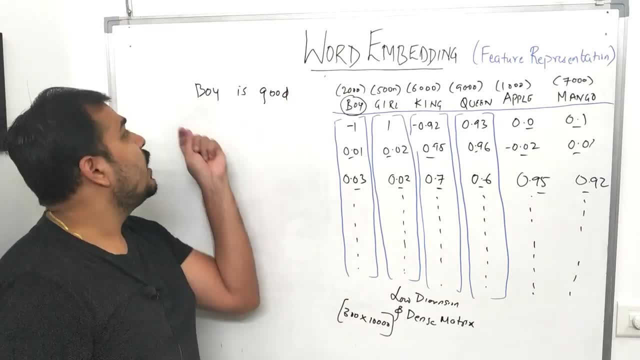 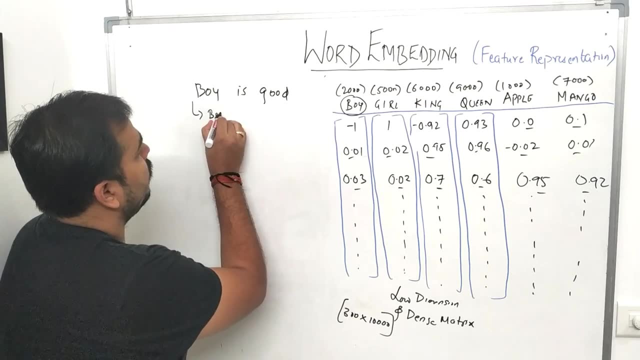 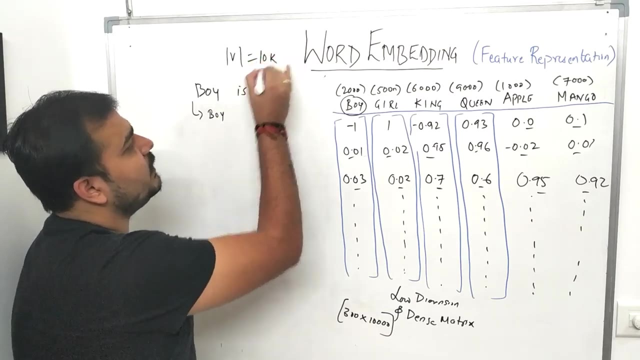 sentence. Now, with respect to each and every word in the sentence, we will try to convert this into vectors like this: How it is done: First of all, let us take boy word. Okay, now boy word. if we first of all will consider a vocabulary size, Suppose my vocabulary size is around 10 K words, Right, 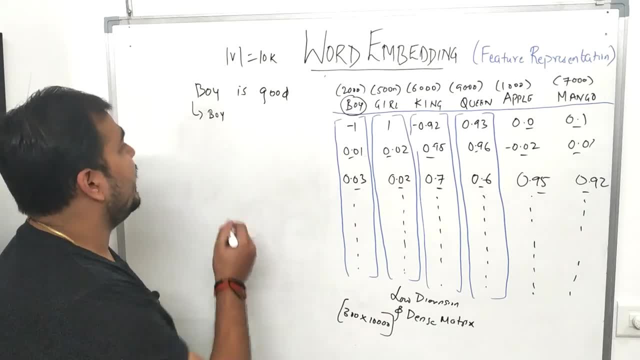 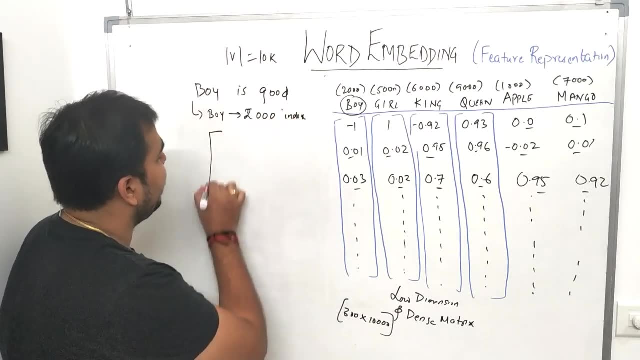 This is the dictionary. Okay, It will be in the sorted order Then for this boy. suppose I have one hot representation of boy. Okay, One hot representation basically means every value will be zero, but at the index 2000 the value will be one. then everything will be zero. Okay, And the? 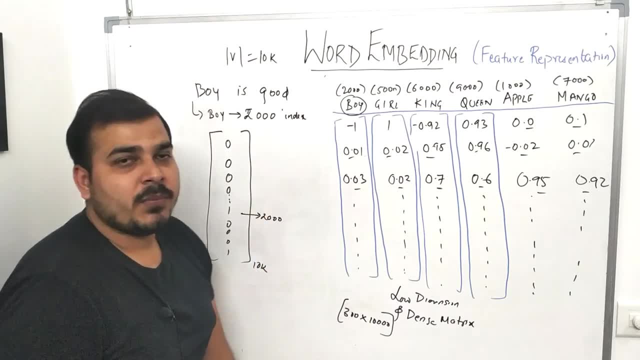 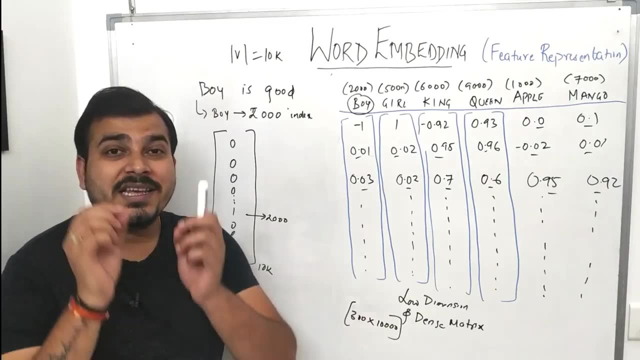 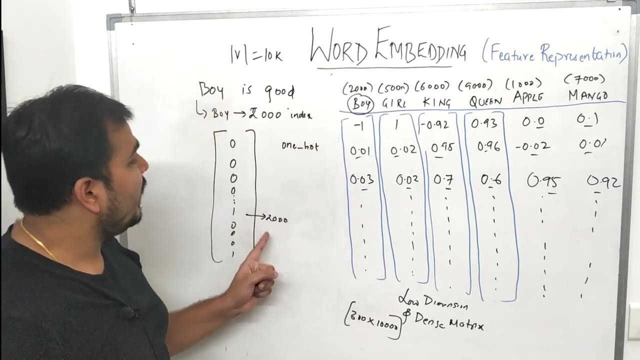 size. total size is 10 K dimensions. Right Now, considering this particular one hot representation, when I apply one hot representation on boy, So in Keras we have a function which is called as one hot, you know, which will actually help us to convert this word into a word. 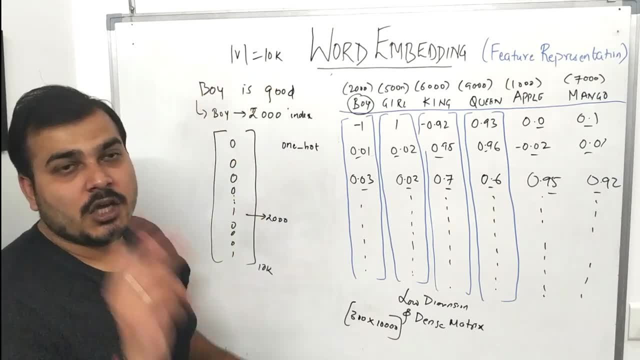 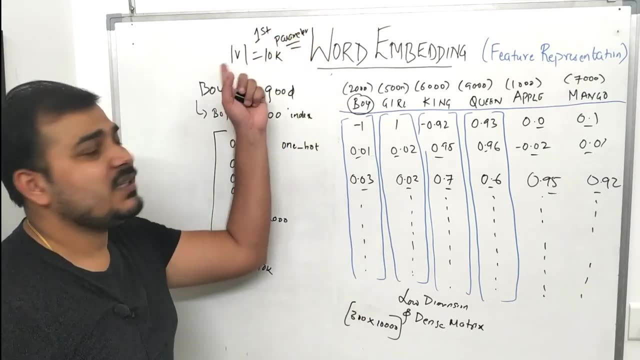 One hot representation considering some vocabulary size. So the first parameter you should remember, guys, is the vocabulary size. Please remember this because in the coding also I'll be using this kind of parameters. you know, I'll be defining some vocabulary size based on the vocabulary side. 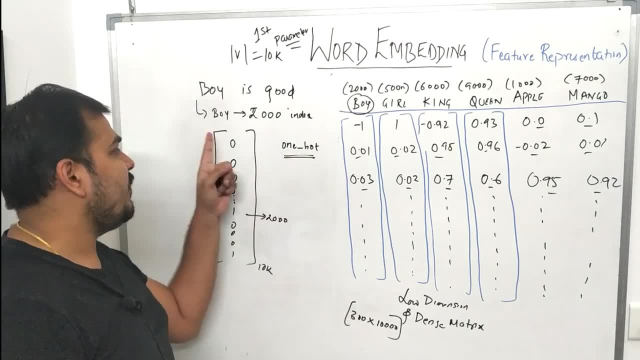 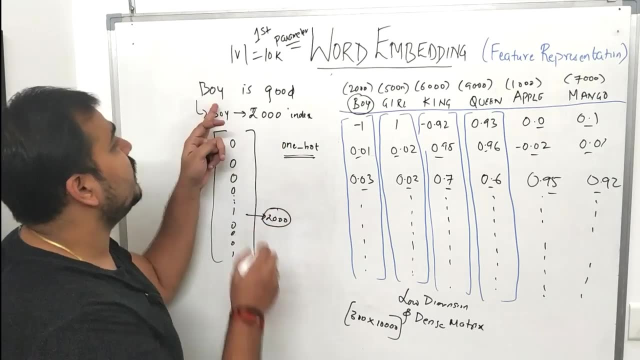 With the help of one hot function in Keras. what I have done is that I have converted into a vector representation. Now, when I do this, one hot will just take out the index number. it will assign some index number of boy based on the vocabulary size. Now suppose in this particular case, 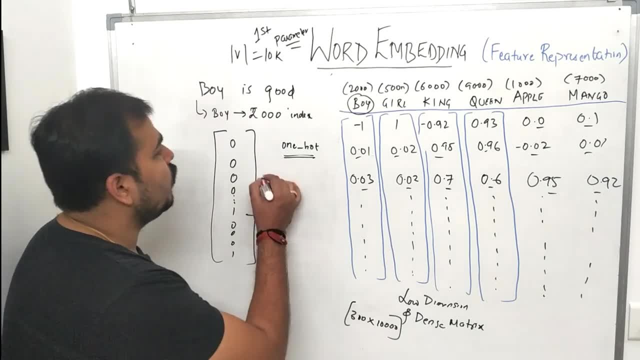 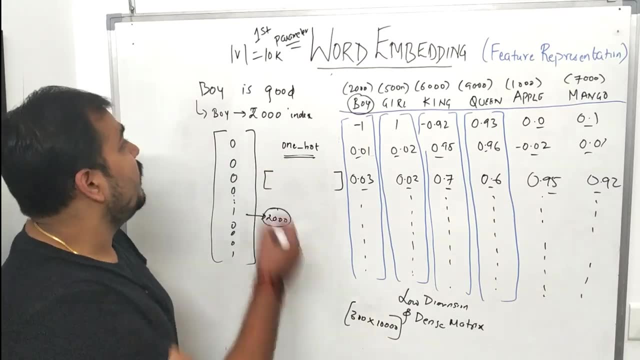 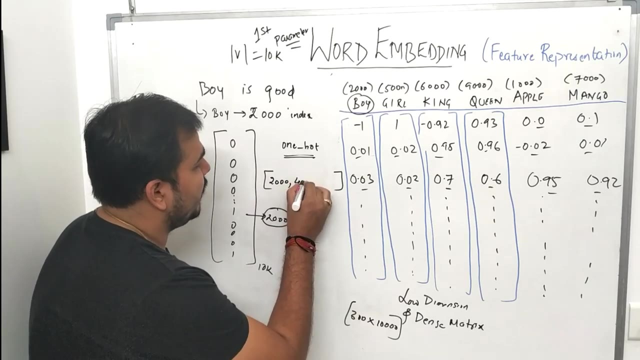 Boy is given. the index number is 2000.. Okay, So the output. you'll be seeing that after one hot representation, one hot representation, basically when it is getting applied for the boy, we will be getting a 2000 index for the ease word. Suppose ease word is present in 4000 index. I'm just taking 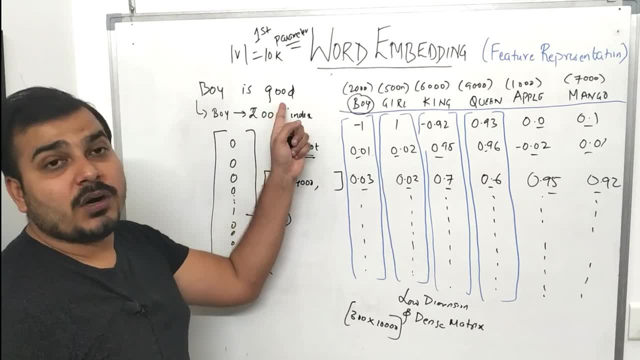 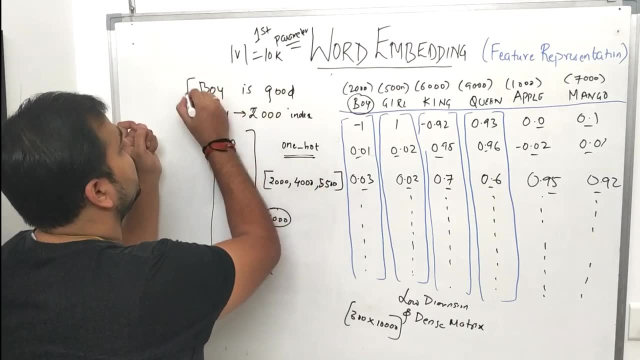 an example: in this vocabulary size as 10 K Suppose, there is a word called as good and this good is actually present in somewhere around 5500 index. So this whole word, this whole word, If I apply one hot representation or if I try to apply this one hot function, I will basically be getting 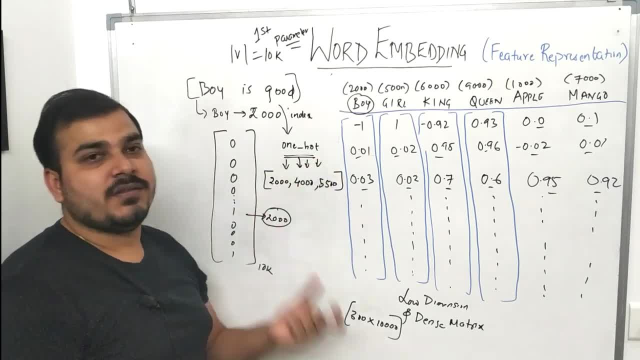 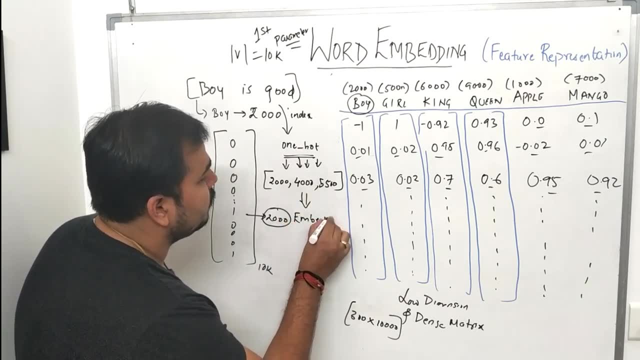 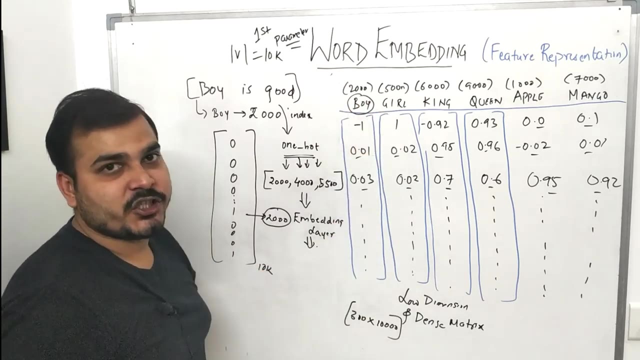 an index of this value. Okay, I'll be getting the index of this value. Now what we'll do is that we will pass this whole value with respect to the embedding layer. Embedding layer, Now, embedding layer. main task is to actually convert this into some kind of vector representation. Now, here I have to give one. 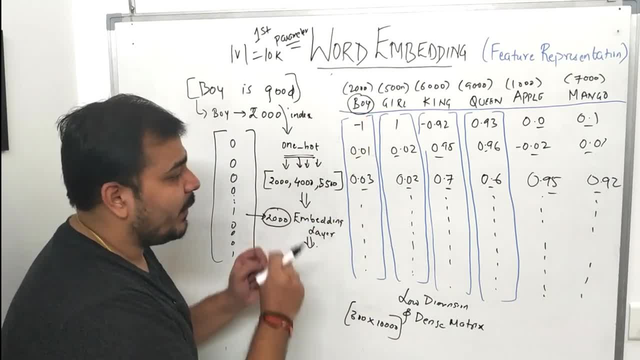 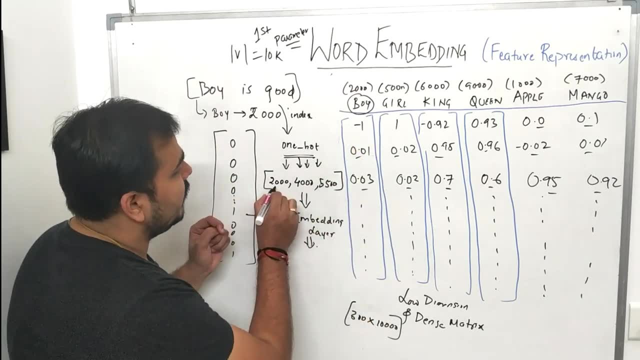 more parameter. The first parameter that I have to actually give an embedding layer is about how many dimensions I want to consider. Suppose, if I give 300 dimensions, that basically means each and every word will be represented in 300 dimension. If I give 10 dimensions, that time, 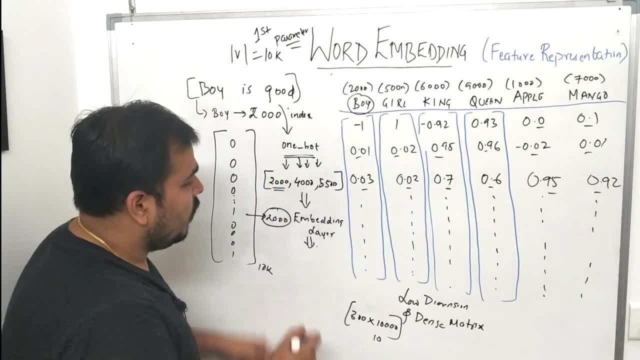 each and every word will be represented in 10 dimensions. So here I will be providing my dimensions. Okay, How many dimension I want? Suppose I'm giving in 10 dimensions, that basically means this whole word, this word of 2000 index, which is nothing but boy. you know it will be. 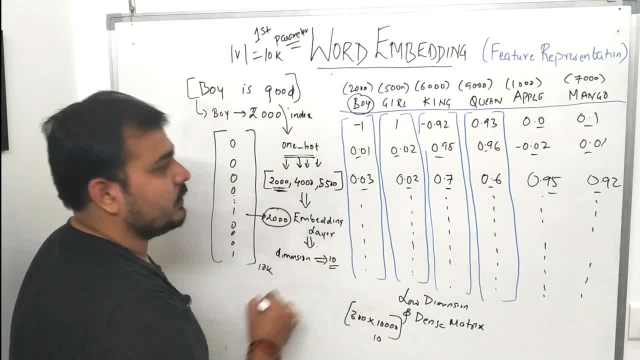 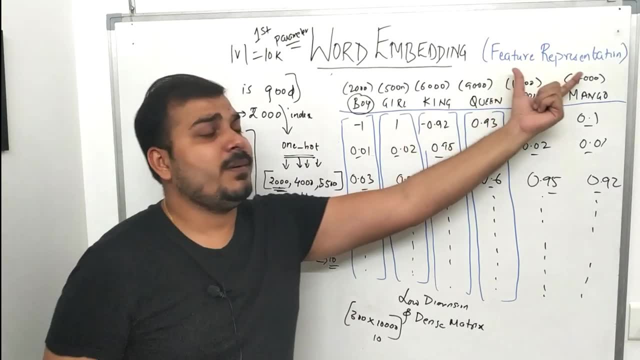 converted into a vector of 10 dimensions. Okay, So like this, I'll be having 10 values and that is the work of an embedding layer. and understand, guys, this embedding layer is nothing, but it is presenting, it is actually creating a feature representation of this particular specific word, Right? So similarly, 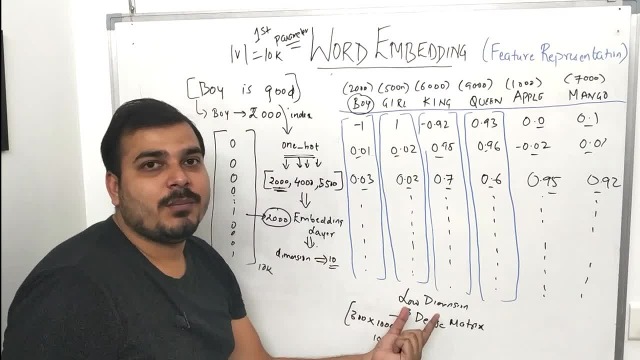 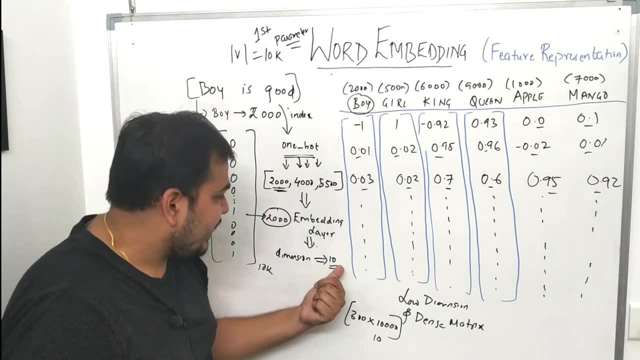 for 4000 index, another 10 vectors of numbers will be coming over here. for 5500 index, another vectors of 10 dimensions will be coming over there. Okay, Suppose, if you take 300 dimension, 300 dimensions will be coming. So I hope you have understood the basic difference This. 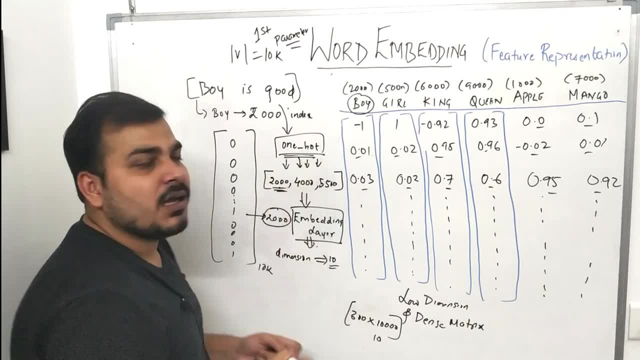 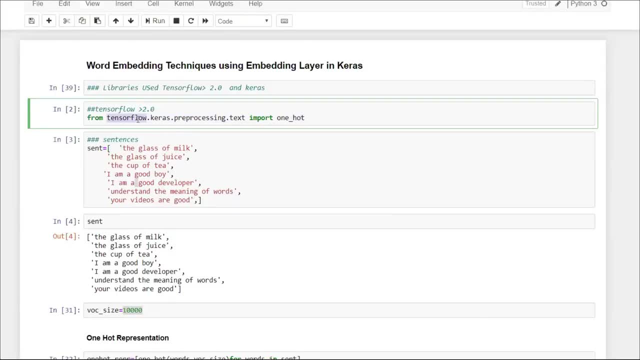 embedding layer is also present in Keras. one hot is also present in Keras. Now I'll go ahead and try to understand the practical part over there, Okay, So let's go ahead. So, guys, before moving ahead with this particular video, first of all I want to discuss what 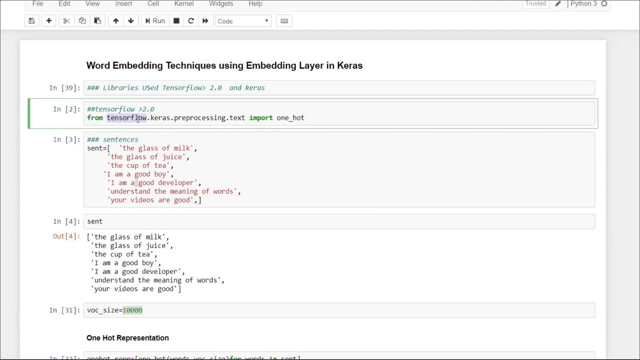 are the libraries we are going to use. So the libraries that we are going to use is Tenselflow 2.0 and Keras, so greater than I. have installed the TensorFlow, which is greater than 2.0, and apart from that, I also have the Keras library. Now, what is the basic difference? 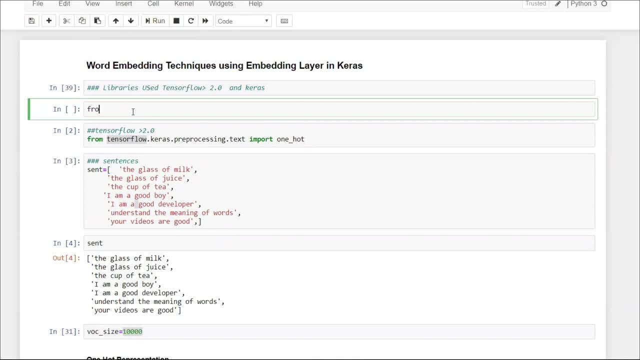 flow less than 2.0. so, guys, if you want to basically import keras, you know um, if you have tensorflow in the back end which is less than 2.0, you can just write from keraspreprocessing: okay, dot text, import one hot. suppose this is just an example. i'll tell you what all this library. 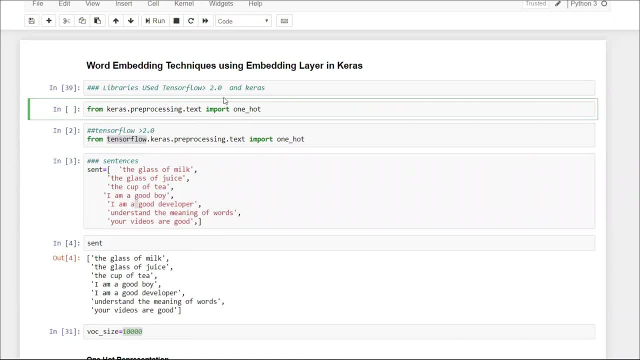 are actually doing now? the basic difference between the tensorflow which is greater than 2.0 and less than 2.0 is that in tensorflow greater than 2.0, you have keras integrated within the tensorflow itself. okay, so you, every time, you will be seeing that we will be writing the. 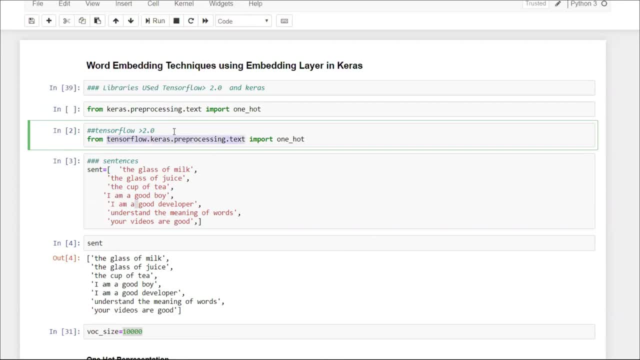 keras library, something like this. okay, so considering this, you can actually execute the program, but if you have tensorflow less than 2.0, you have to write your libraries like this. okay, you have to import your libraries like this, but you have to install the tensorflow also. you. 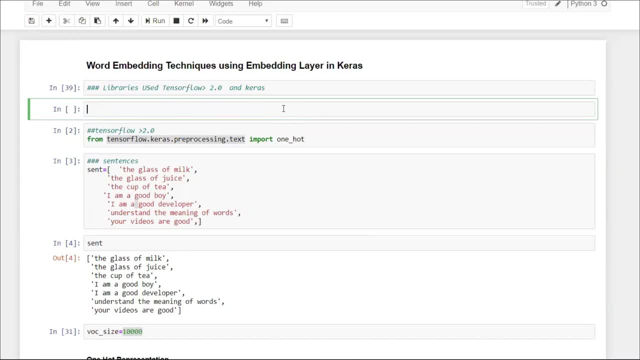 have to install the keras also. so here i'm going to consider an example where i'm showing you how to do that, and i'm going to show you how to do that in a little bit. you with respect to tensorflow greater than 2.0. now, the first thing is that, as 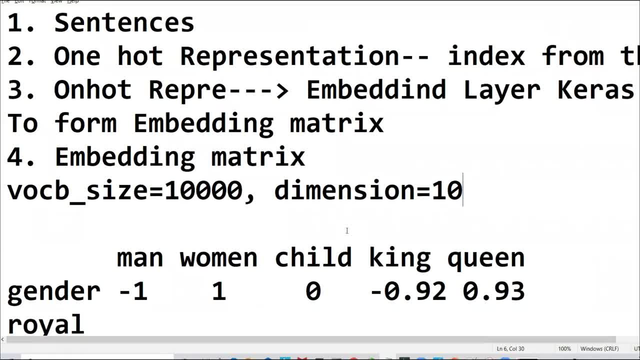 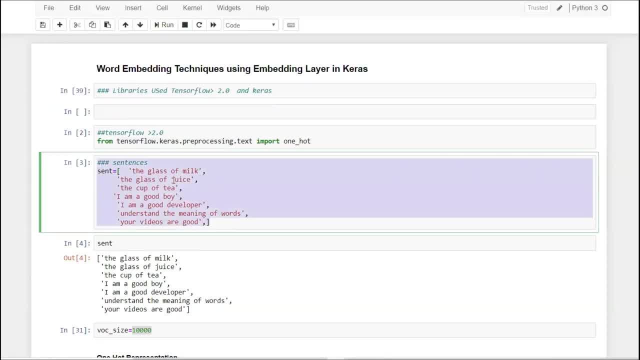 I told you from this particular excel sheet, in sorry, this particular notepad, is that I am going to initialize my sentences. so here is my sentences. I've taken a simple example of all the sentences, like the glass of milk, the glass of juice, the cup of tea. I'm a good boy, I'm a good developer, understanding. 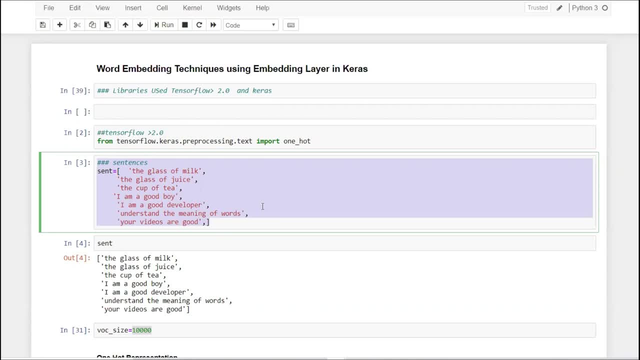 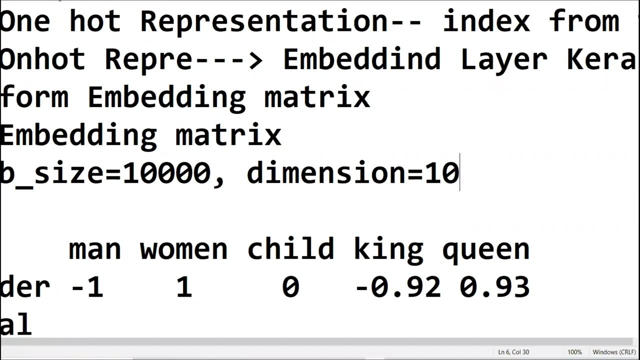 the meaning of words. your videos are good, so these are the basic example of the sentences. in the next step, what I am doing is that I will actually form a one-hot representation- ok, one-hot representation- of this sentences. so let me, let me see how we can attribute. for that, you will first of all require a. 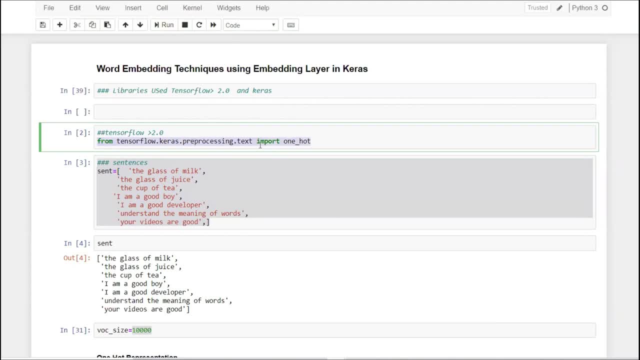 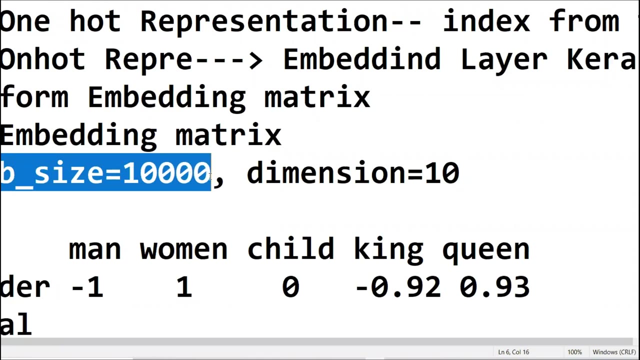 library. ok, from tensorflow, dot, garage, dot, preprocessing, dot text import 1, underscore heart. so this is the library which we have to use for actually converting this particular sentences into one heart. ok, but before that we need to initialize a parameter which is vocab sighs. vocab sighs basically says: 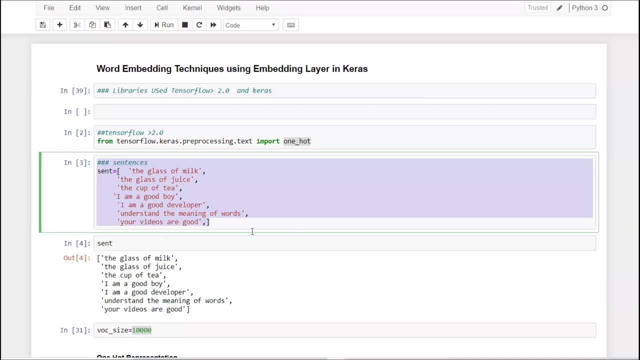 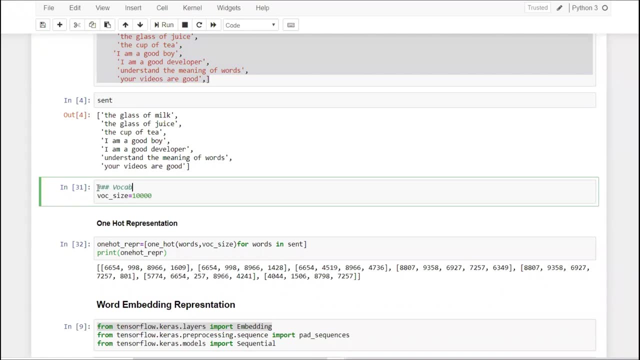 that what is the size of the dictionary? ok, considering this, what I have done done is that here you can see i have actually initialized this vocab size, so i'm just going to write a comment over here. this is my vocabulary size. vocabulary size. okay, now, once i have the 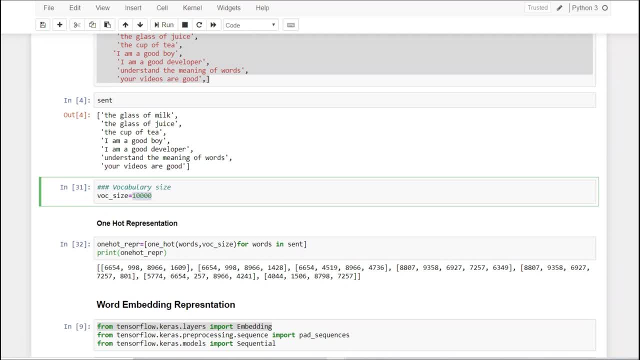 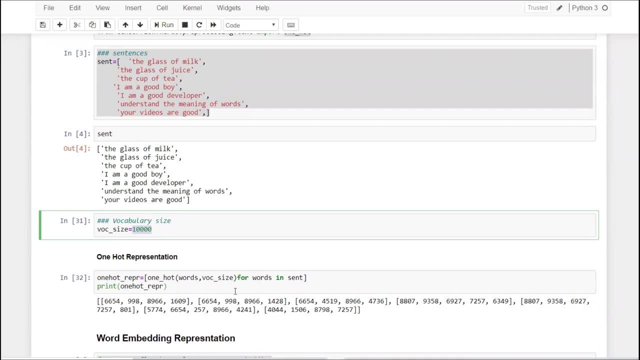 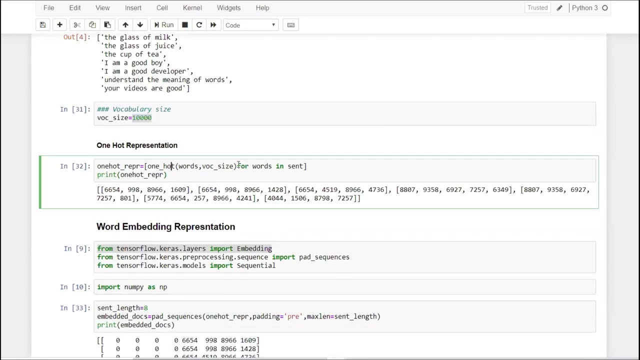 vocabulary size. this is my ten thousand now now. now, see, very important thing is that how i'll be converting the sentences into vector, into one hot representations. so for that, what i'm going to do is that i've already imported one hot, so i'm just going to write this particular code. so for words, 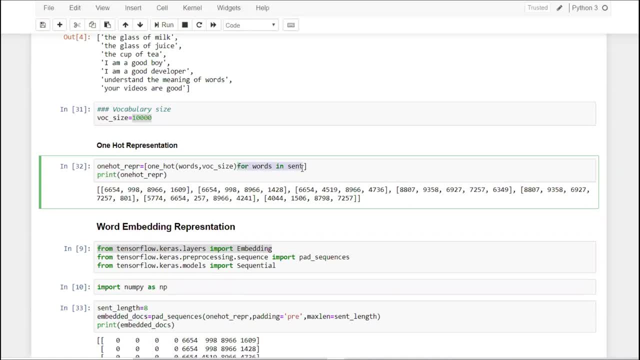 in word for words, in sentences. that basically means for each and every sentences. it is traversing through each and every word. i'm going to pass these words to a function that is one hot where i have to pass word and the other parameter is basically vocab size. okay, so this basically takes. 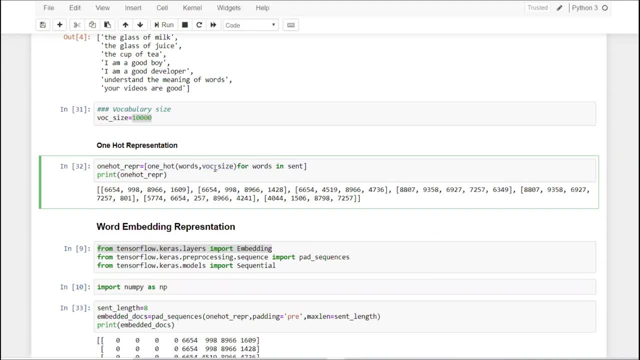 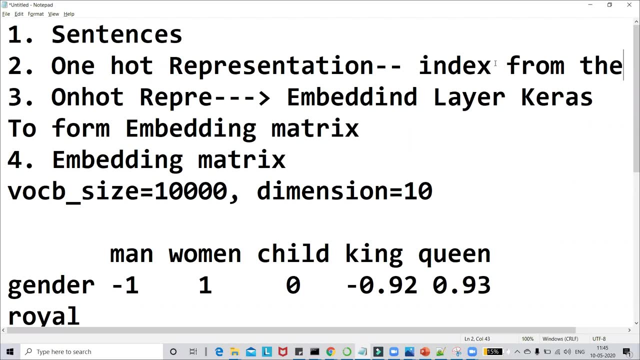 the word, which is the word and, with respect to that, what is the vocab size? and based on that, it will provide you an index. so we will be getting the index. remember this: we'll be getting the index from the dictionary, right from the dictionary. we'll be getting the 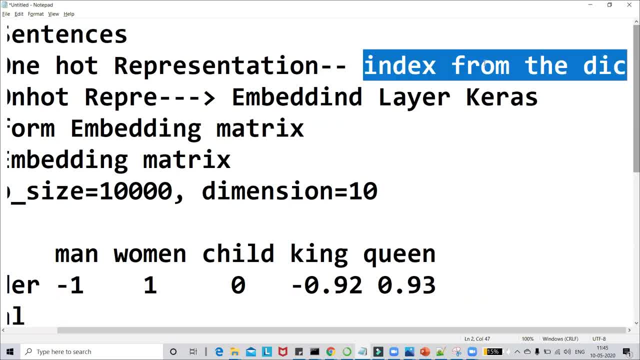 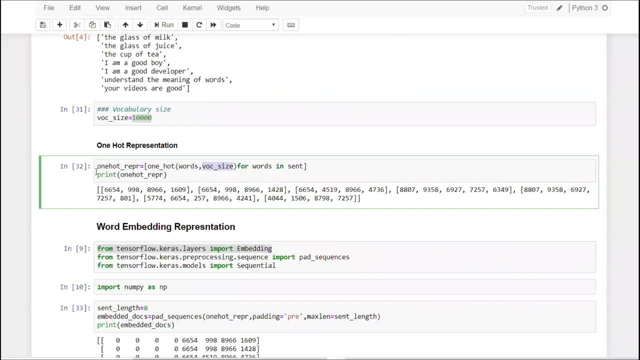 index here you can see. i've written it clearly. we'll be getting the index from the dictionary, okay, and it is treated as like a one hot representation of it. so as soon as i do this and if i'm printing the one hot underscore representation there, you can see that for each. 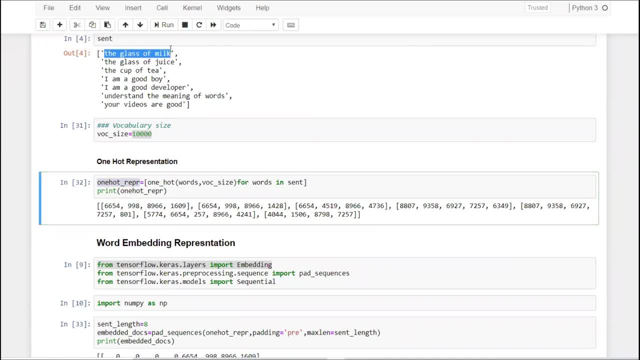 and every sentences, so first sentences is like the glass of milk. now, here you can see: the index is six, six, five, four out of that ten thousand vocabulary size, and always remember all these numbers that will be coming, it will be less than ten thousand. the second number, second word, is glass. okay, then, glass is basically having the index of nine, nine. 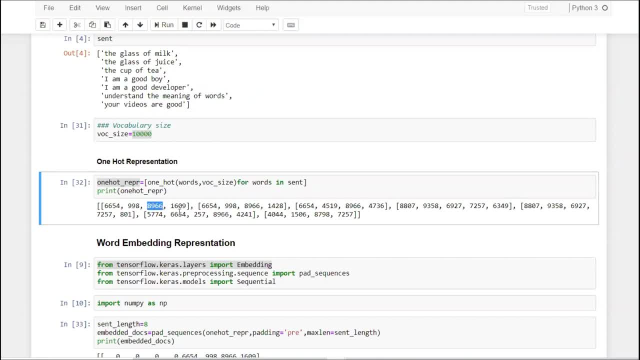 eight. the third word is off. it is having eight, nine, six, six. the fourth word is milk, so i'm having the index as one, six, zero, nine. now, a very important thing to note over here, guys. you can see that the first and the second sentence is almost same. only milk and juice is different. right, but you can see. 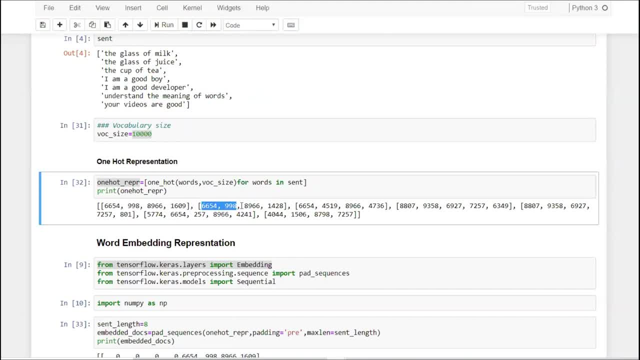 over here. that basically means this: three words should match right. these three indexes should be matching. you can see, over here we are having six, six, five, four, nine, nine, eight, eight, nine, six, six. here also we have: we are having six, six, five, four, nine, nine, eight, eight, nine, nine, six, eight, nine, six, six. okay, so both are matching. only this last index is matching. 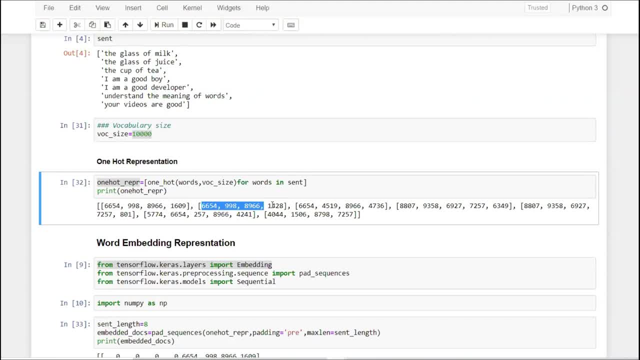 so this is how you have actually got this particular index representation- pretty much simple, and that was explained in my theoretical part also. i noted all the points in my notepad also. now, considering this, what i'm going to do is that the next step? let's, let's go to the next step. 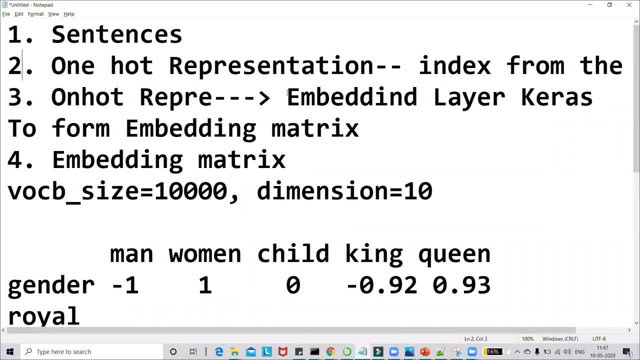 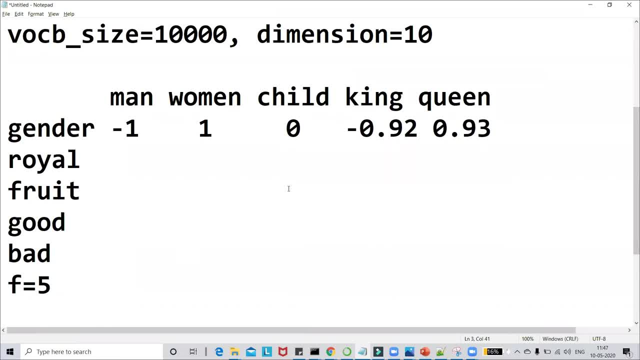 now, whatever one hot representation i have, i'll be passing through the embedding layer in keras to form an embedding matrix. embedding matrix basically means this kind of matrix, right, this kind of matrix. now, one important parameter for this is that how many dimensions i have to give that, basically, how many features i have to get right this, this, because it is a feature. 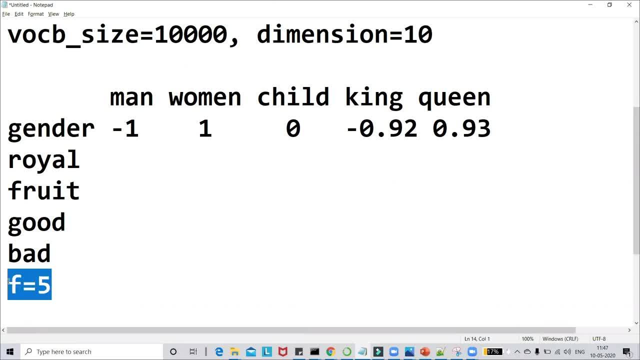 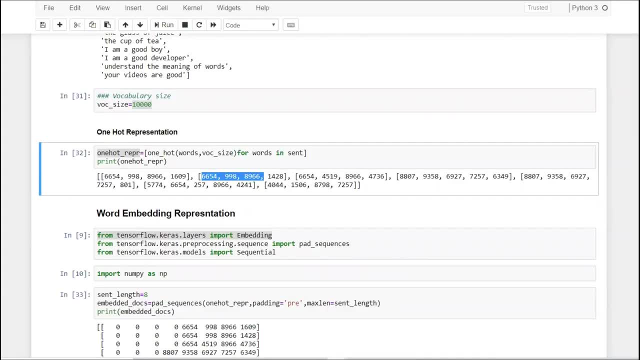 representation. suppose i have here five features, so i'll be giving my dimension value as five. okay, now let's see. before that, we also have to do one more important thing. let's see what is that. now, what i'm going to do is that i'm going to import embedding layer. 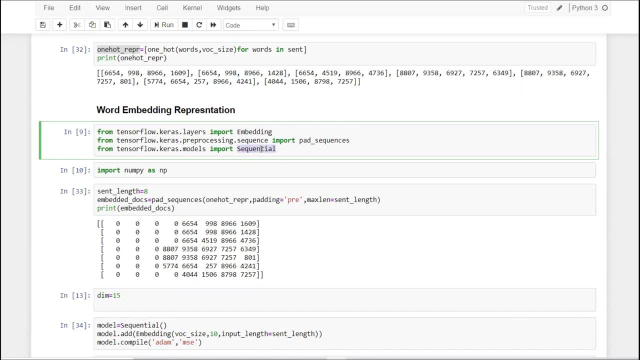 i'm going to import the sequential layer because, uh, we have to use a sequential model in order to create uh with respect to the embedding layer itself. so over here we are. we are going to initialize the sequential model. for that, you just import first of all the embedding layer. 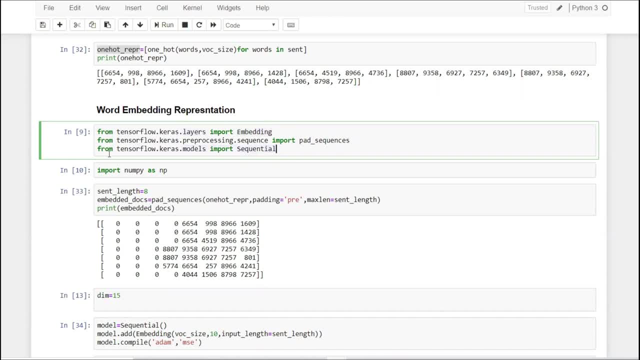 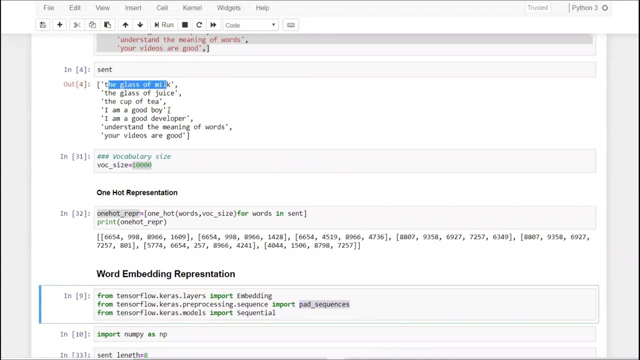 from tensorflowkeraslayers: import embedding. then here you can see that i have imported sequential. then, apart from that, there is also something called as pad underscore sequences. now why this is so important. understand, guys. whenever we want to pass anything to the embedding layer, all the sentences should have the same number of words, because that will actually help us to create. 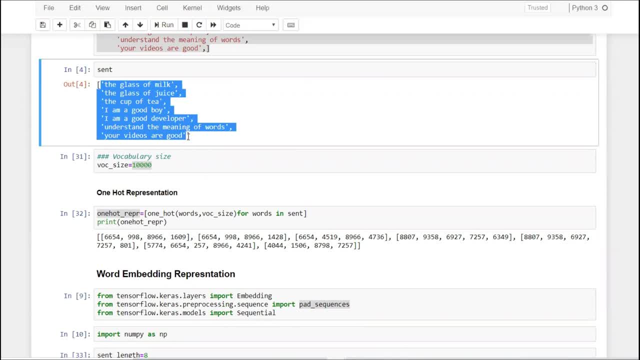 a very good embedding matrix right, so that since in lsteam in the future, you'll be seeing that whenever i'll be implementing the lstm, at that time i'll be using these pad sequences too much. you know more than we'll be using many types, so at that time you can see that we will. 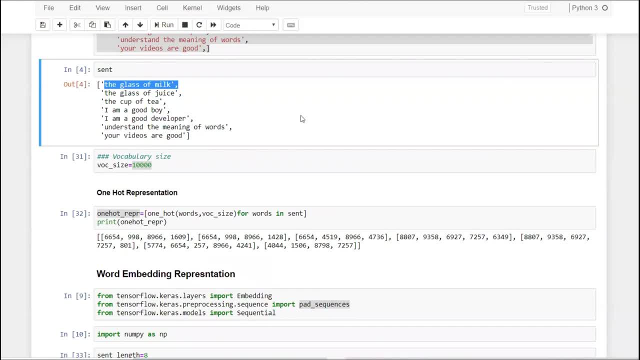 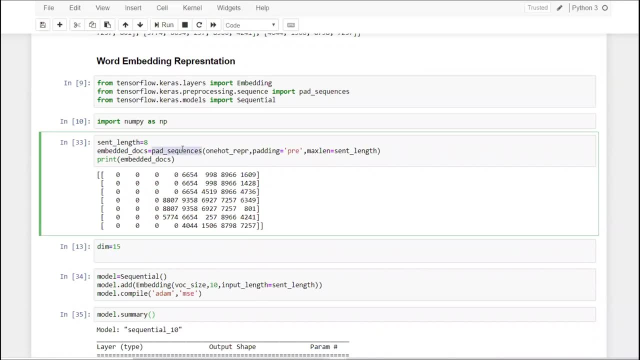 be passing these particular words and make sure that the size of the sentence is the same and for are actually using pad sequences. now understand in pad sequences what all parameter goes on. okay, so in pad sequences, first of all, i have to provide what is my one hot representation. 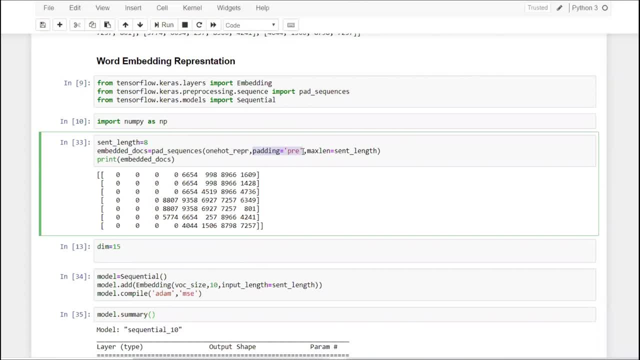 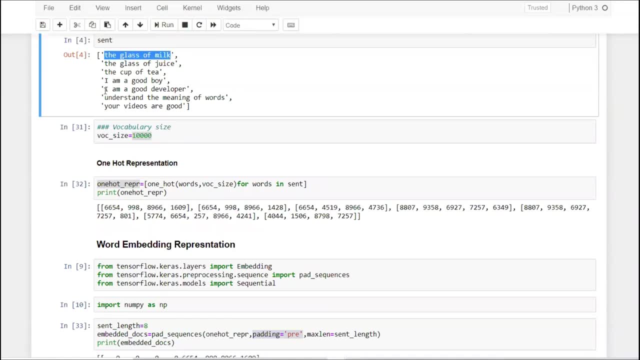 and what is the padding technique? now? what is this padding technique? guys understand one thing. suppose you can see over here i have four words, over here i have five words over here. now you can definitely see that there is one extra word here. there is one less word now. if i want to make 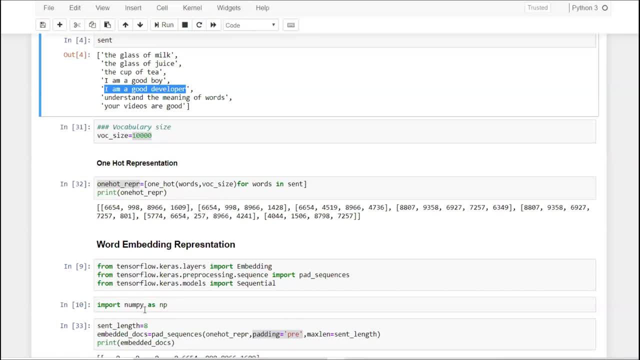 this word of the same size. first of all, i will say that what is my maximum sentence length i want? okay, so that i can add padding on top of that. so i'll say that make all these particular sentences of length 8, so that it will be fixed. i can change it to 10 also, and based on the problem statement. 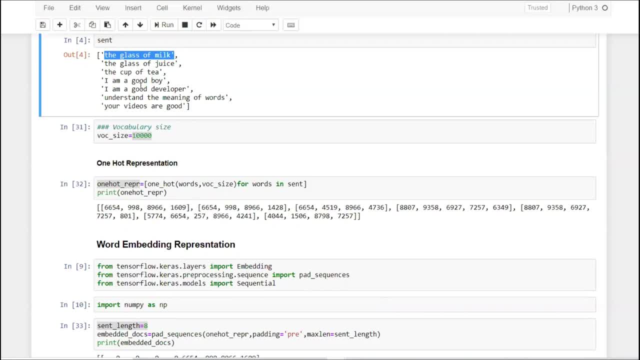 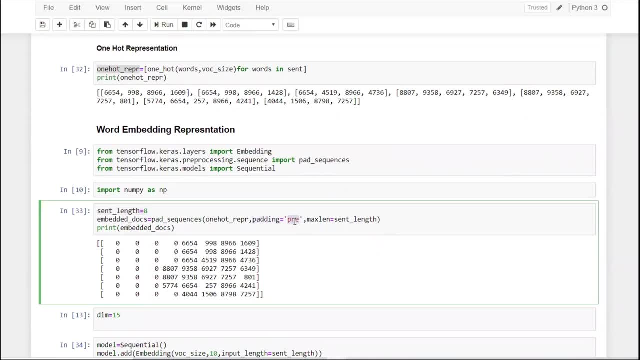 you can vary that particular parameter, okay. so when i'm doing this, here is one parameter which is called as padding. okay, this padding will actually- and if i give the value as pre, it will add zeros in the front and try to make the sentences a complete eight word sentence. okay. 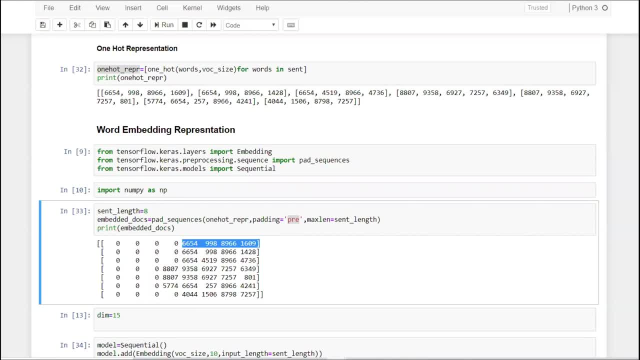 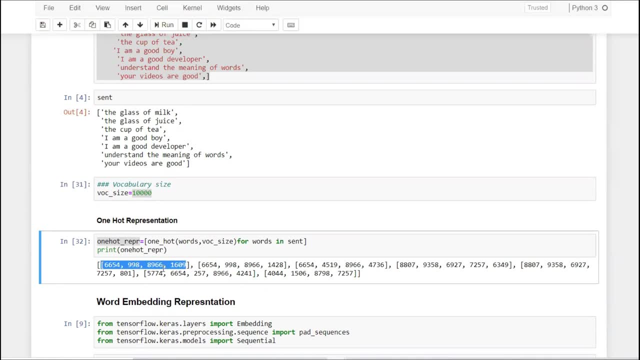 now here you can see. this is my four words initially, which i had in my first sentence, right the glass of milk you can see over here. this is my glass of milk. now this is still four words, but i have to make it eight words, and here i'm using the padding technique as pre. so what it? 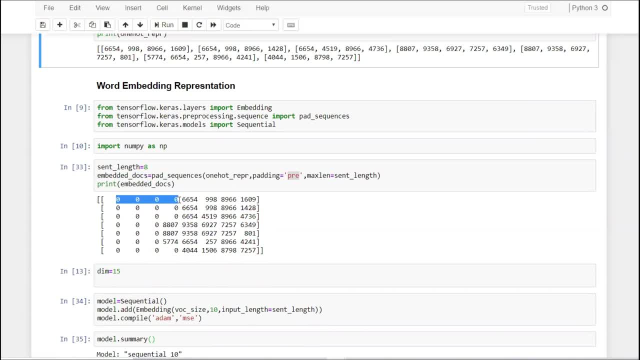 is going to do remaining four words index. it will add zero, zero, zero in the starting point starting from here. so that's the padding technique. similarly, you can see here i had five words and it is getting added three zeros in the front. three padding has actually happened, if i change. 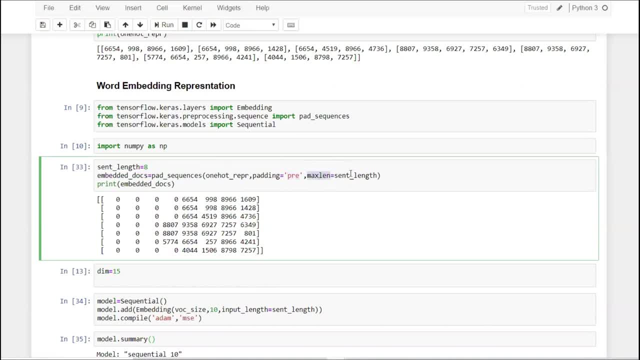 this into post, that zeros will be added at the last, and you can see that i have also given the maximum length which will be my sentence length, that is, of eight. so by default it has converted all the sentences over there to the eight word sentences. so that is what we have done and this: 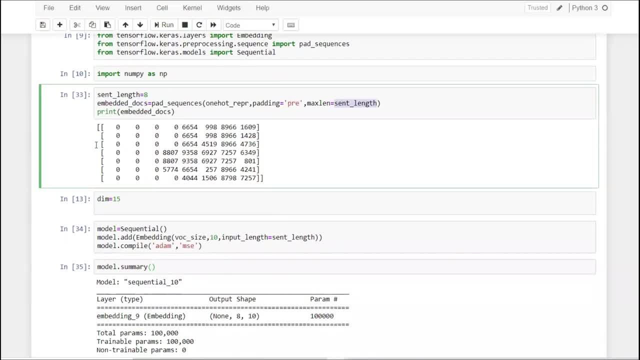 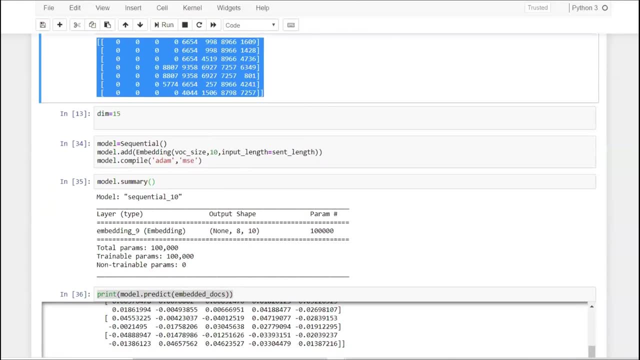 is a very necessary steps when we are actually working with lsd. now let's go to the next step. i'm going to pass this to my embedding layer now. in order to pass it to the embedding layer, i told you, first of all, we have to consider that dimension. suppose i've taken the dimensions at 10. 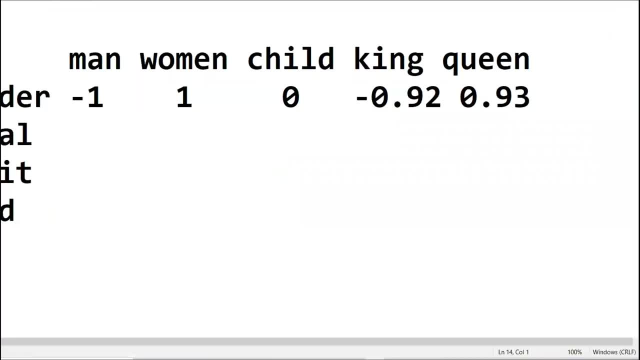 okay, dimension, basically, is that features, this, this features, right? how many features? uh, how we are to go ahead with the featurized representation, how many dimensions i have to take, right? so i have taken 10 over here. in this particular example, there is five. okay, now the next step is that i 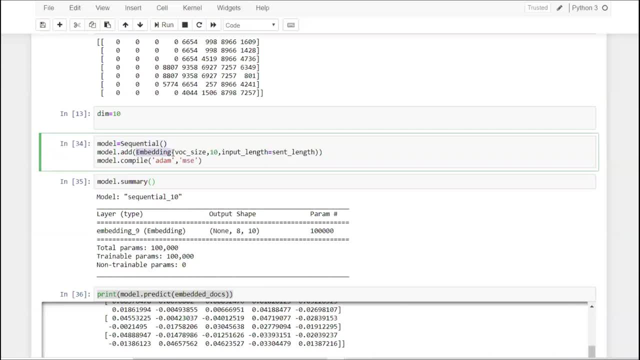 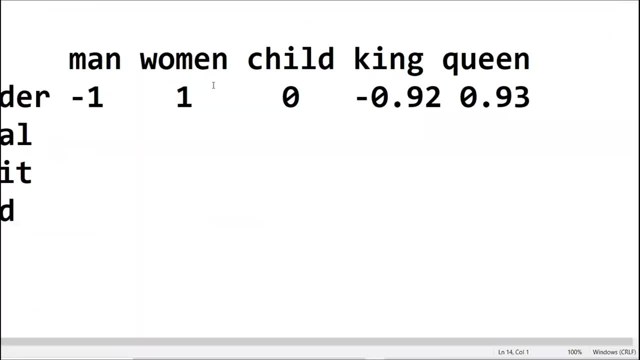 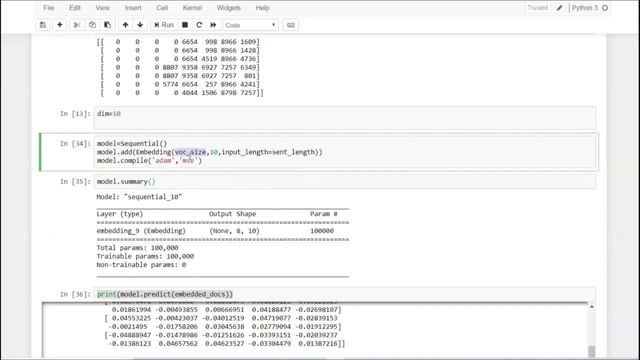 will be adding a dimension to the dimension model, then i'll be adding an embedding layer. now, this is pretty much important. this embedding layer actually helps us to convert, based on the number of dimension, into a feature featureized representation, like i've shown you in this particular example. okay, there, the first parameter is basically a vocabulary size. okay, remember the. 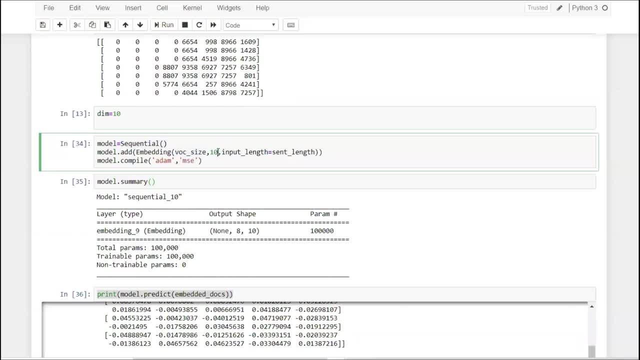 first parameter what i'm giving vocabulary size. i told you the second, the second parameter, is our dimension. okay, these two are vocabulary size and dimensions. this is pretty much important, so i'm going to give our sentence length. sentence length, how much we have actually taken over here. 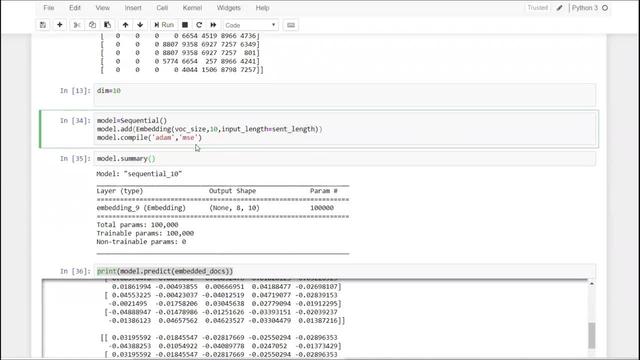 somewhere around eight. that's it once we add this embedding layer, and then we will actually compile it with the adam optimizer, considering the performance metrics as mean squared error. and when i write model dot summary, you can see that this is basically my model dot summary, pretty much simple. it is having an embedding layer right now in order to see how my words have actually got. 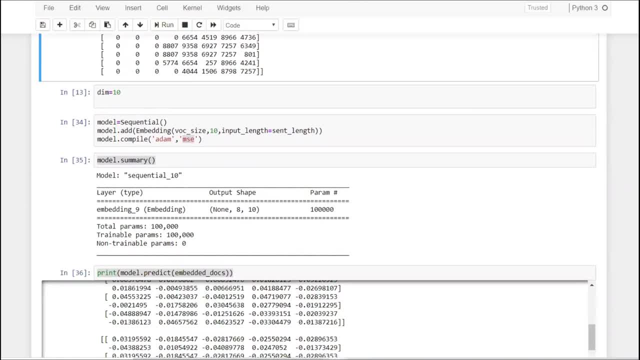 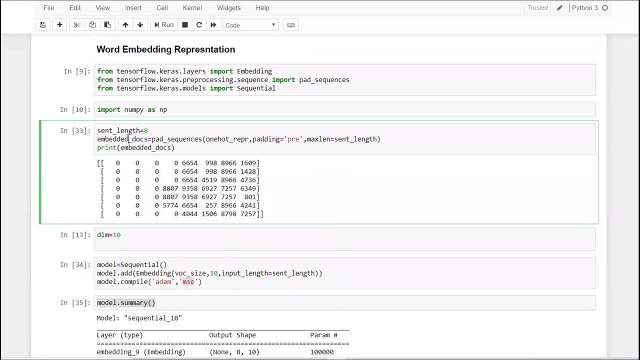 converted. how suppose this particular word has got converted into featureized vector? we just have to do model dot, predict. and here i'm just going to give my embedded docs. embedded docs is nothing, but this value, this whole sentence is in form of indexes. so when i give this, you will. 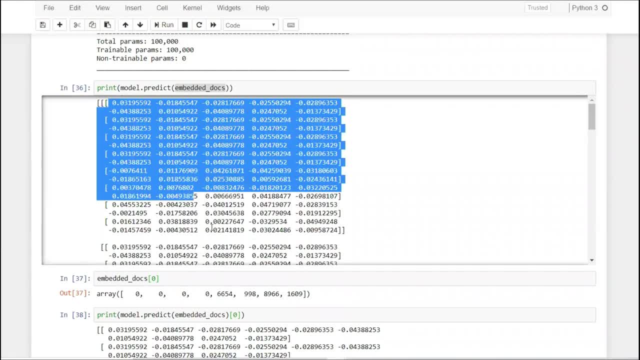 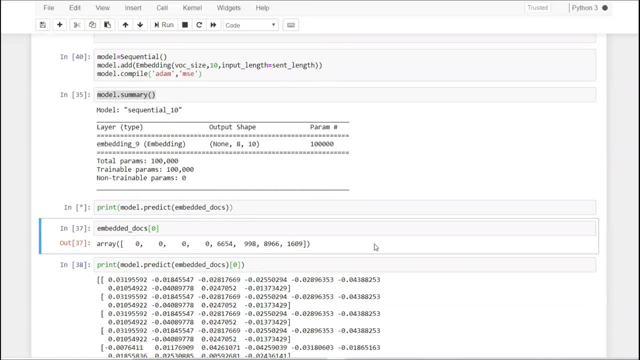 be able to see that the printed value. i am getting this many values right. you can, you can see over here. let me just execute this once again. okay, here you go. okay, fine, perfect, so i have got this. now. probably you'll not be able to understand, uh, because there are. 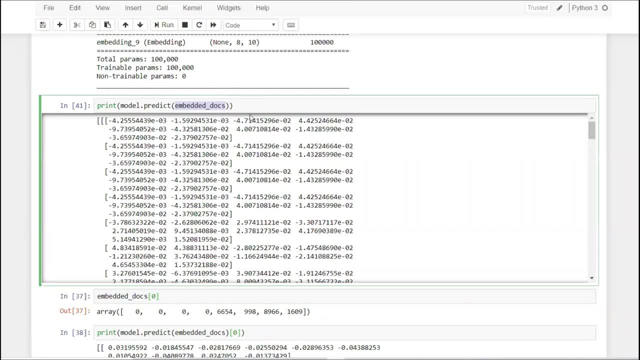 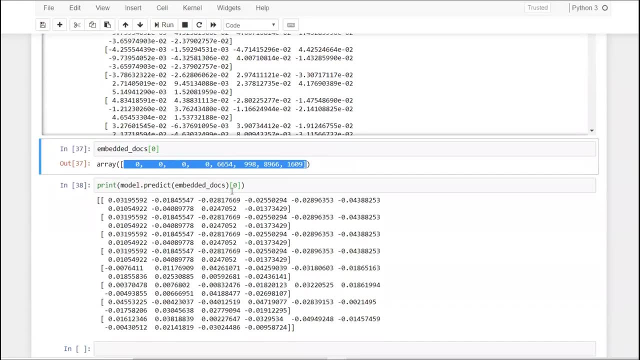 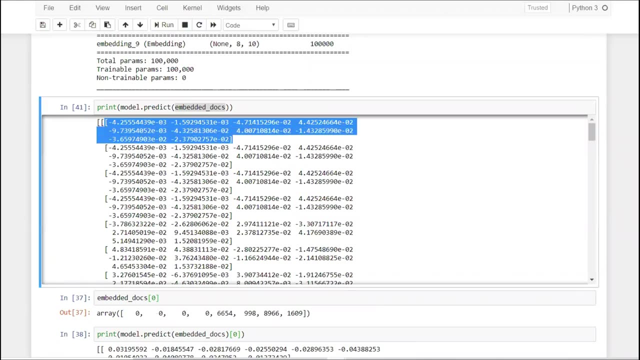 many values. let us do one thing. let us just take embedded docs of the zero. this is my zero first sentence, right, with respect to indexes. now, similarly, whatever i'm printing, i'll be taking this first. i'll be taking this first representation that i've got in form of vectors. okay, so let me. 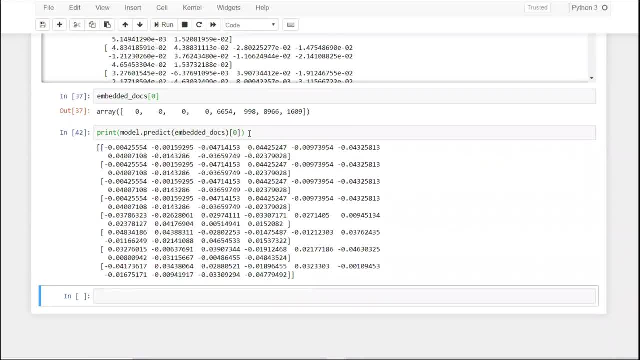 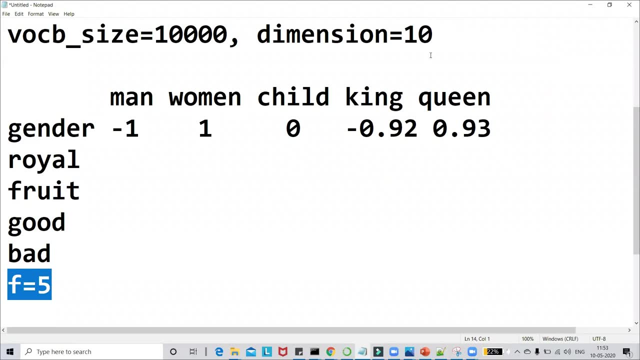 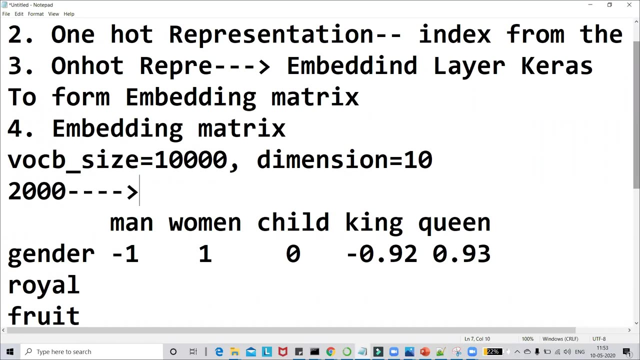 just write this and print this now see what is the important thing over here. i told you that the number of dimensions that i am going to take over here is 10, right? so that basically means if i'm giving an index of 2000- okay, this is my word- this will get converted into a dimension of 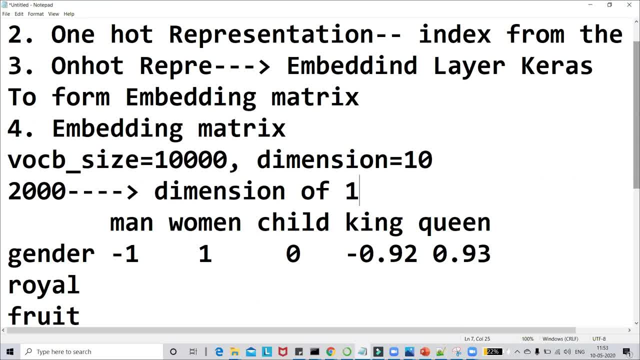 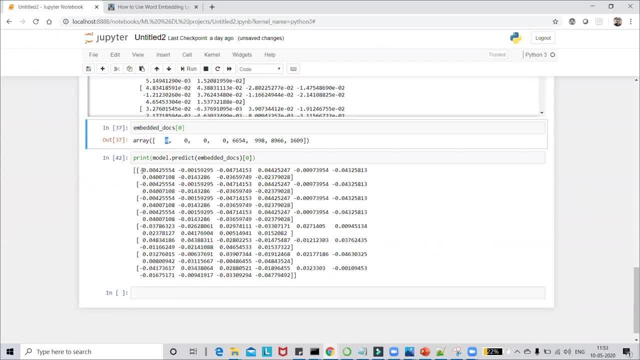 dimension: dimension of 10 vectors. right, 10 vectors. now just understand this. zero has got converted into a dimension of 10 vectors, so this is my one: two, three, four, five, six, seven, eight, nine, ten. i have literally counted in front of you to make you understand: these are 10.. 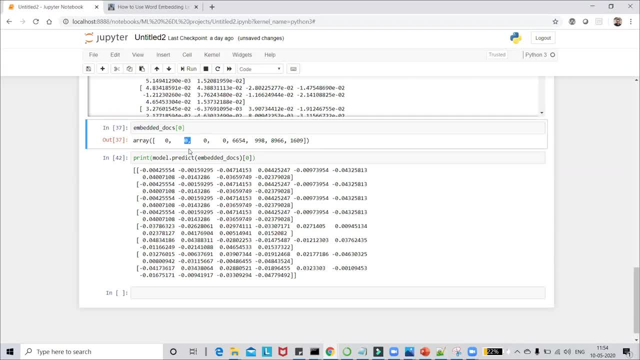 now let's go to my second word in the same. this is my first sentence. right now i'm going to the second word in my first sentence. so here is my first second word of the first sentence. right, this is represented again at- and i'm uh- 10 dimension vectors. okay, now, if i consider this, 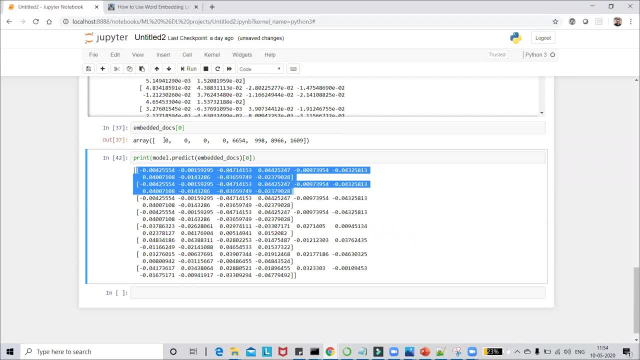 two. these two are same. why it should be. why it is same? because both these values are zero. next value, first four ten dimensions that you will be able to see are having the same value. there is no difference, guys. okay, so this basically indicates that this zero index vector has got zero index.